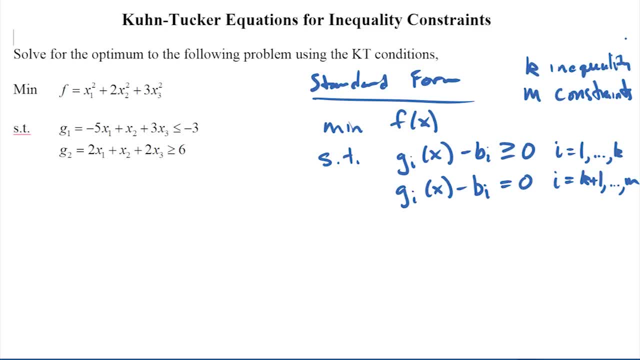 k inequality constraints, and then also in this, I have m minus k equality constraints. So equal sign versus inequality sign there. And now I'm going to show you how to use the equality constraints. And now I'm going to show you how to use the equality constraints. 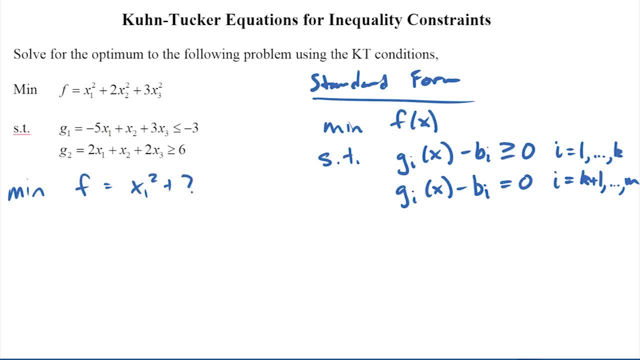 going to take my problem and just transfer it to the standard form first of all. so there's my objective function. it's a quadratic programming problem subject to some linear inequality constraints. okay, so I have greater than or equal to 3, so I just multiplied through by a negative switch. the sign on. 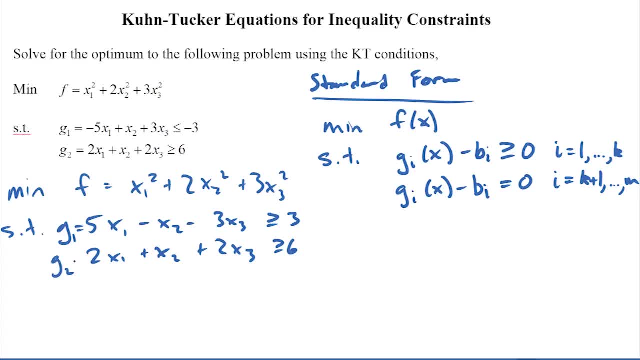 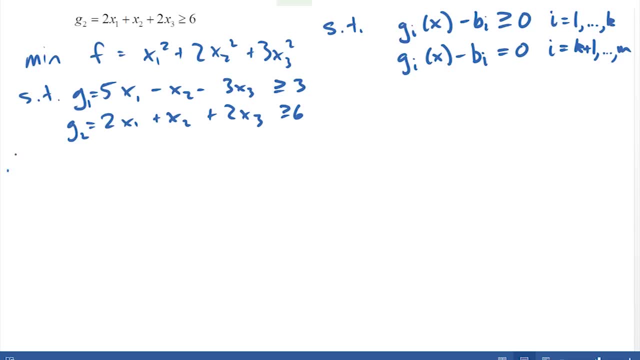 that and put it into the standard form. I have G 1 and G 2, and now what I'm going to do is is I'm going to go ahead and assume that both of my constraints are binding, okay, so that they G 1 equals 3 and G 2 equals 6. so I'm going to treat 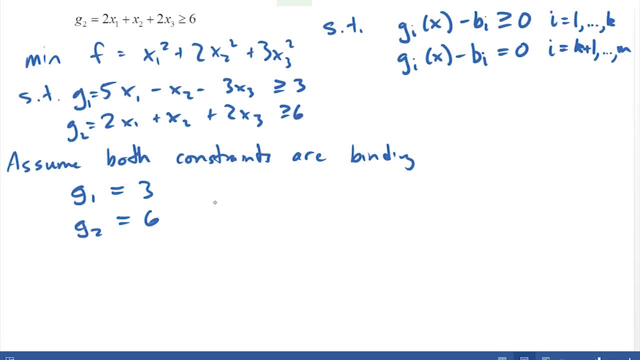 them like equality constraints first of all and then solve this problem and then look at the Lagrange multiplier afterwards. okay, so we can. we can see the sign of this Lagrange multiplier after we solve the problem- assuming that they are binding and that their equality constraints- and see if this is a good assumption that G. 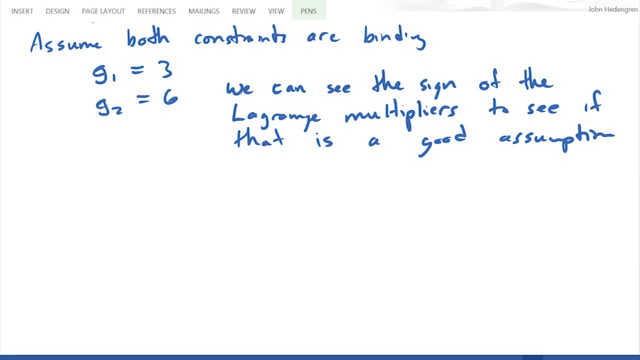 1 should equal 3 and G 2 should equal 6. okay, so I'm going to go ahead and write. write the second from the second conditions of the Kuhn Tucker Krish: Kuhn Tucker conditions. go ahead and write out these equations for each of. 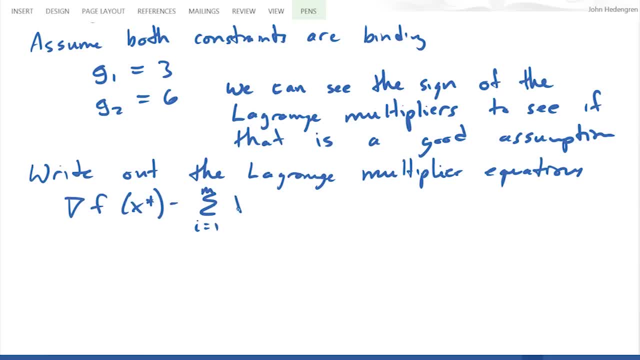 each of these. so I have my second condition for the KKT. I have my gradient of my objective minus the gradient of my objective, minus the gradient of my objective minus the summation of my Lagrange multiplier. the time is my. the criterion of my equations s equals 0. okay, so I'm going to write this out. 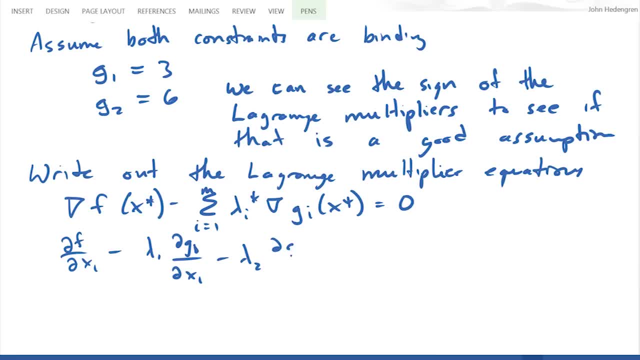 element by element now. so I have, in this case I have the variables X 1, X 2, and then also X 3, and then I have my two equations. so I just have 2 Lagrange multipliers in this example, so Lambda one and Lagrange two, one x two plus X, 1,2x, which is D powers k1 minus x3, and then I have two equations, so I have just have to Lagrange multipliersIn this case so lambda 1 andございます. 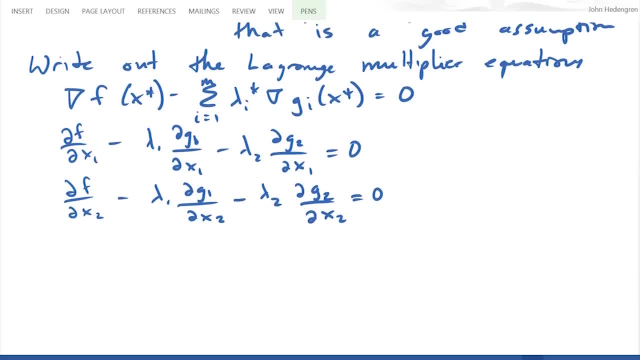 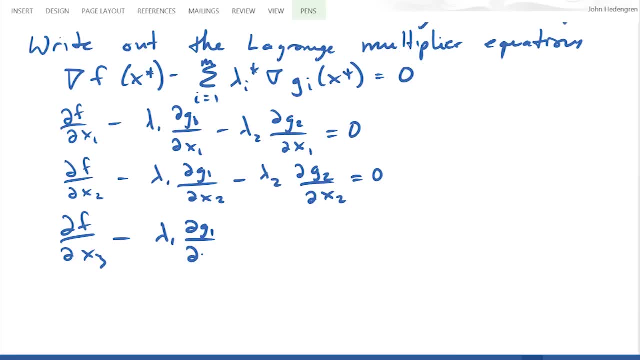 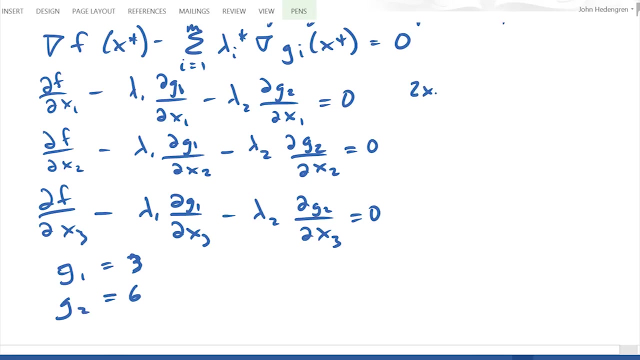 lambda two, and both of those are going to be equal to zero. I'll do my third equation as well, and so this is just with respect to x3. okay, so I differentiate both my objective function and my inequality constraints with respect to x3. x2 at x1, and then I assume that g1 and g2 equal the right hand side. 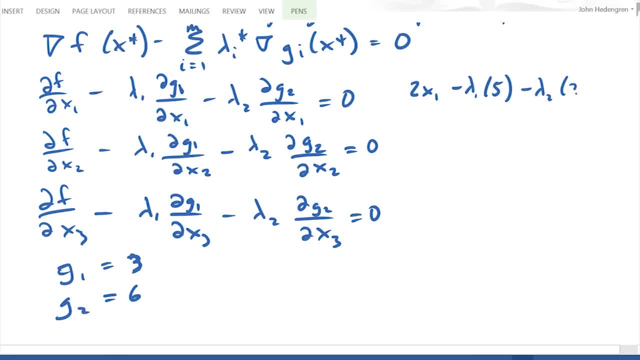 or the B values. okay, so I'm just going to write out these values for for these equations. I'm just going to take the partial derivatives for of the objective function also of the equations and come up with my three equations. so in total I have five variables: x1, x2, x3, and then lambda 1 and lambda 2, and then I can. 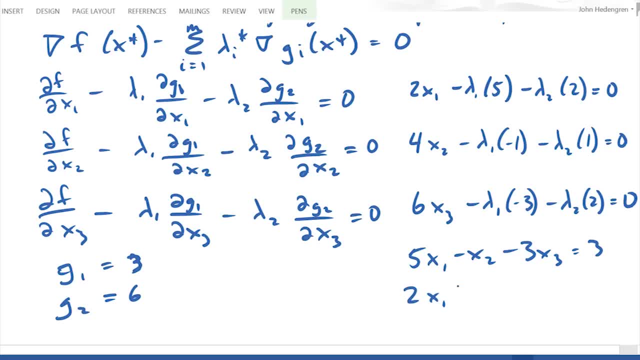 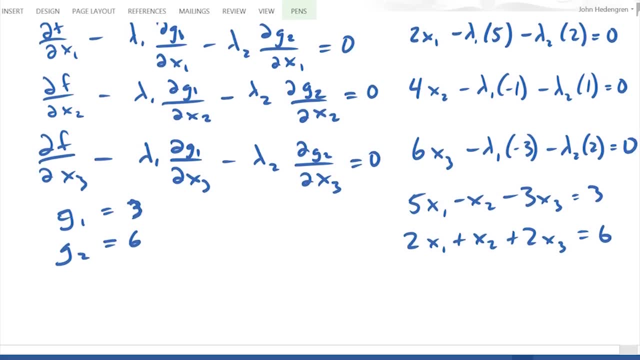 solve this problem by solving a system of equations. the nice thing about quadratic programming problems with kk, kt conditions is that it results in a linear programming problem. so I can just do one inversion of that matrix and I come up with my solution. so there's my solution for x1, x2, x3, and then I'm also have a lambda 1 and lambda 2. okay, so now. 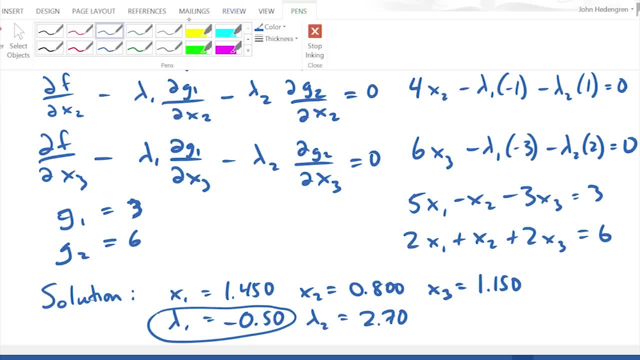 I have my solution. so I look and see that one of my Lagrange multipliers is negative. so this is the fourth condition, the Kuhn-Tucker condition, and this is the fourth condition, the Kuhn-Tucker condition, that is violated. so this is not an optimal, optimal solution. so what do we? 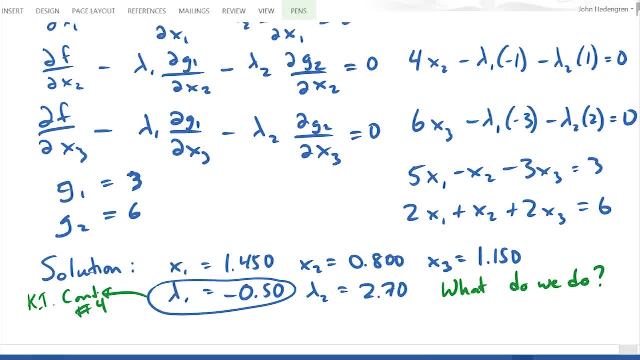 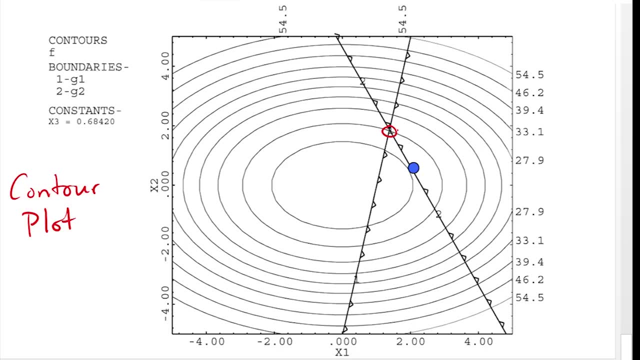 do with this. so so that what you do is the negative of Grunge multipliers is you go ahead and fix the Lagใช kuhn-Tucker Grace multiplier at zero, so it's not at the, it's not a binding constraint, and then drop that constraint. so if the optimal solution were here on the contour. 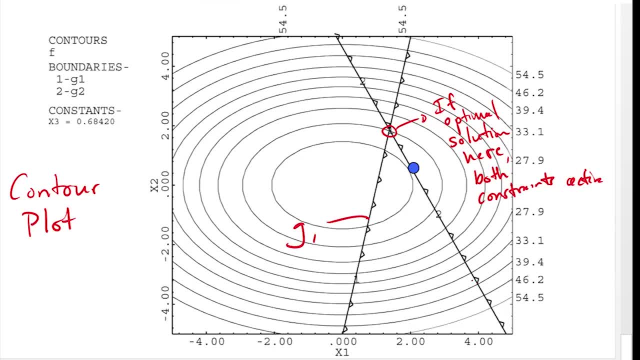 plot, then both constraints would be active, the blue dots actually being active. so that makes up for the negative canción here. if you look at this case, say I've got my blue dot value and then I've got delta x5 and then double delta x5. now I have the super Matte and the point of course I got delta x5 and then 2 of them are consecutive. so in total we can divide the same thing. 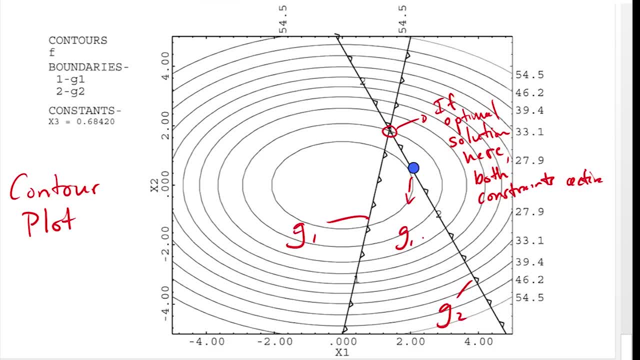 The blue dot's actually the optimal solution. There I have my G1 and G2 constraints and you can see that G1 is not active at the optimal solution. So what I'm going to do is just set lambda 1 equal to 0 and resolve.